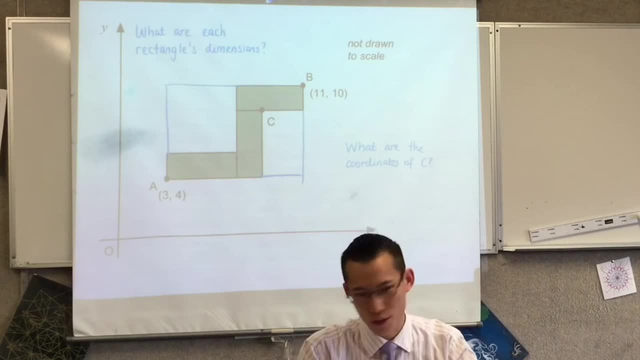 too, but I'm no chef. I'm no chef. I have no understanding of, like, what flavors are supposed to combine together. what if you get given a mystery box and there's just these random ingredients and then you have to think of something that will bring them all together? why do you put an oven at 180 degrees and not like 250? 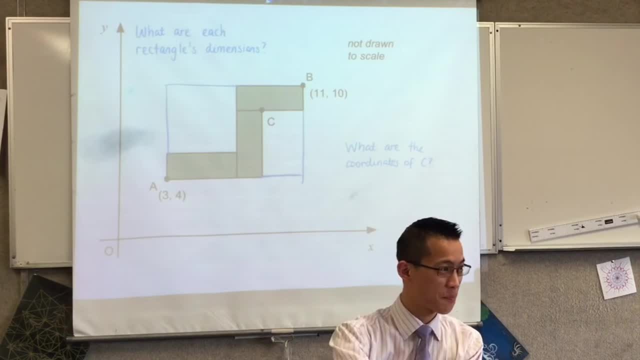 degrees. I can tell you which one you should do if you've got a recipe, but I don't know why. I don't know why you add cream of tartar. I don't even know what cream of tartar is, but apparently it's important right now when you look at 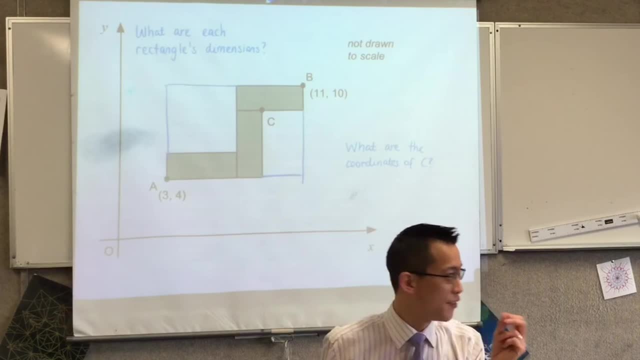 this question. you look at this question. I'm convinced, if I've done my job all year, that you guys know everything you need to know in this question, but you're not sure how to combine them. so first thing I'm going to notice is: look at the. 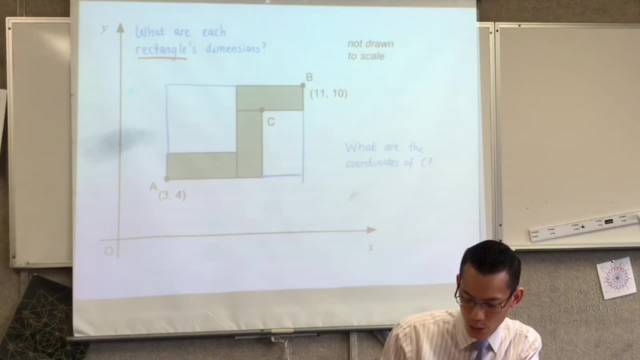 question. take it one at a time. it says what are each rectangles dimensions? so that's like, how wide, how high are the rectangles? right now I don't know what those numbers are. there's two numbers I'm trying to find and don't know what they are, but lucky for me, I have a whole. 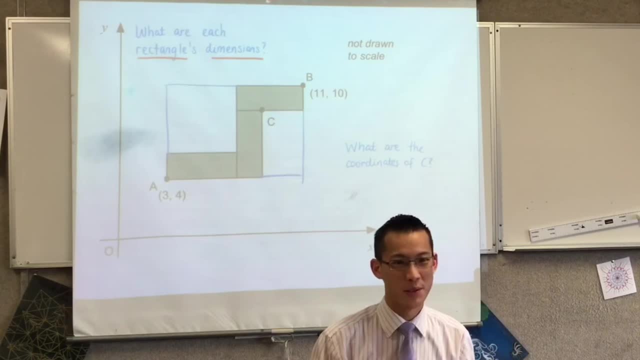 branch of maths that's all about working with numbers when you don't know what they are. what's it called? it's called algebra, right? so the question never says: use algebra. but I look at, I'm like, ah, this is a great question where algebra can help me. I want to know the width, I want to know the height. so I'm gonna use 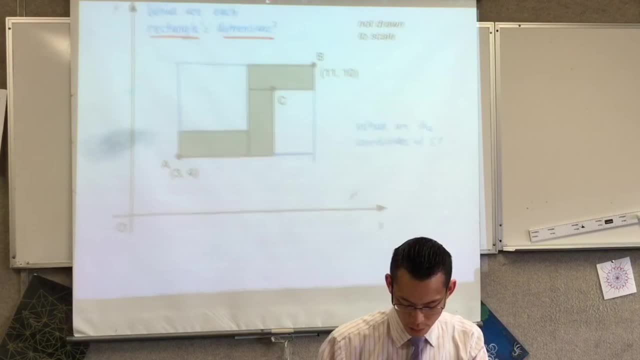 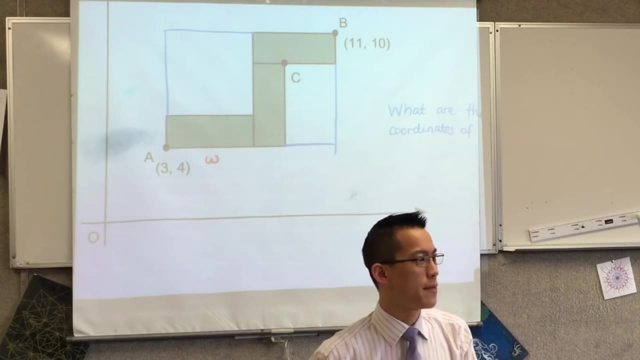 algebra. I'm gonna give each of those a name, okay, so, for example, let's have a look down here. I've got A's and B's and C's. I'm gonna say, well, width, I'll call that W. maybe you want to add on to your diagram that you've drawn there there's. 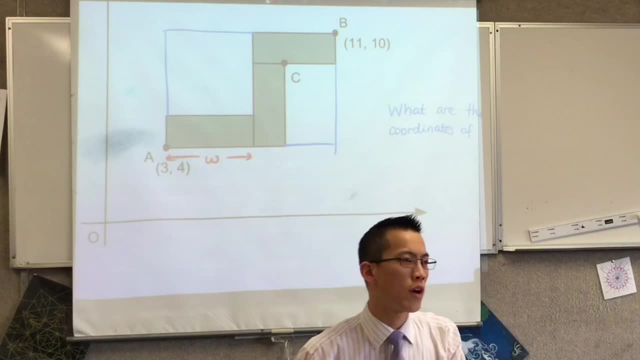 the width across this way of one of the rectangles. okay, that's the width. I also got how tall the rectangle is, how high it is, so I'm gonna call this thing over here H for height. okay, so I've got a width, I've got a height, I don't know what. 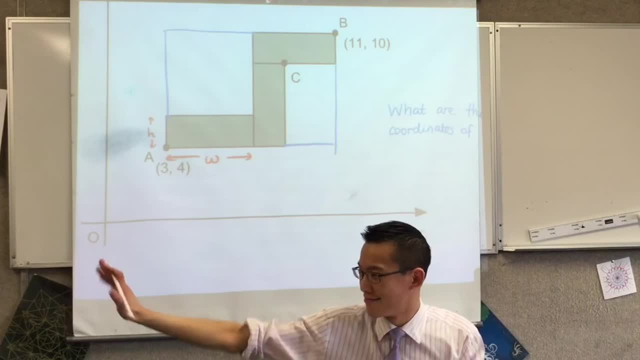 they are right. but that's okay, stop, you can wait now. the wonderful thing about giving these names is now I can see where they are right. I've got them over there on the bottom left, but where else can you see W and H? where else are they? yeah? 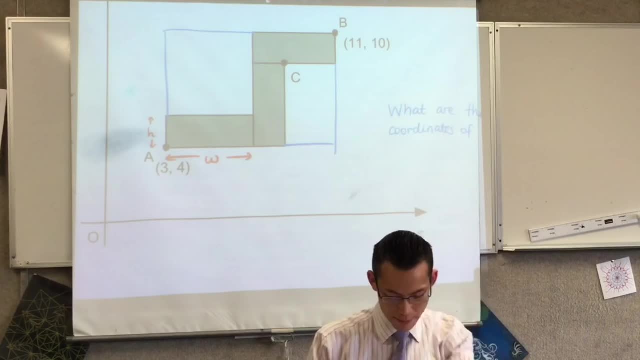 turn on on the top right, right next to me. there's another W this way and there's another H this way. right, that's good, but remember, you also know all these rectangles are the same. so there's one more place, or one more pair of spots where you can see W and H, can you see? 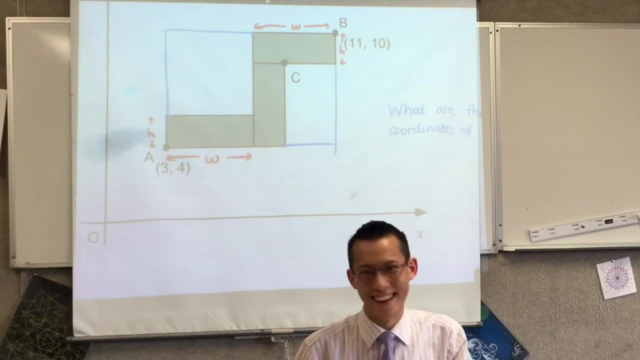 them, no, the, they're a bit so helpful to kill. okay, you can see this spot here, right, what's that? that's a trait. and this one here, this is W. right, it's the same one again. do you see it? do you see it? cuz the same rectangle? it's just been. 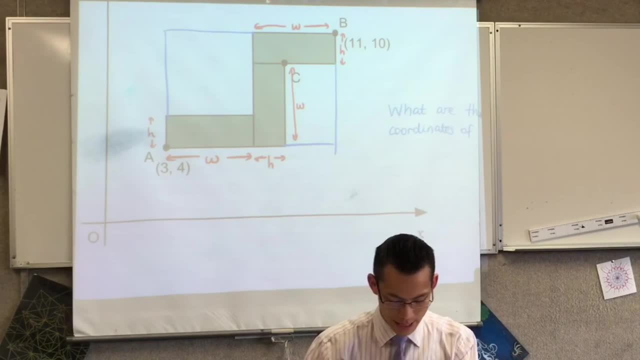 moved around. okay, now, what is that? All right, now, I'm almost there. I'm almost there. You know how I drew those blue lines. They're kind of like those scaffolding things that help you out. right, I said that was my clue. 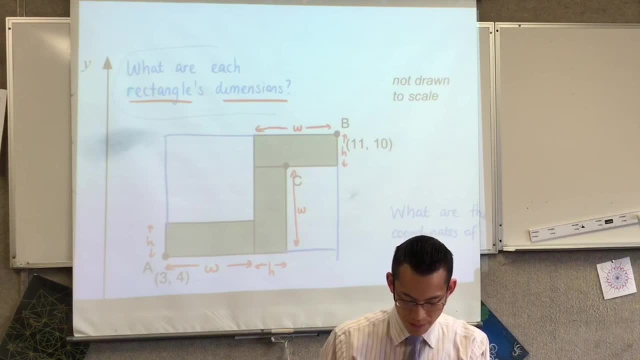 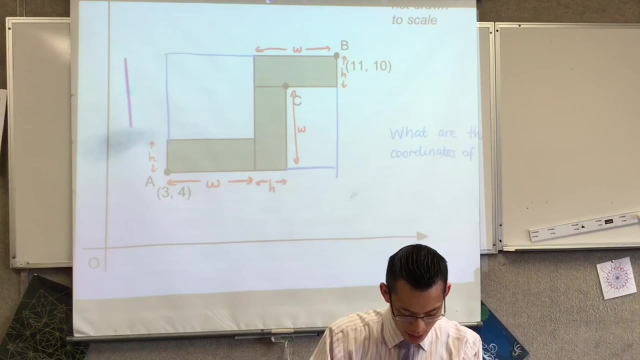 Now, whether you realize it or not, let me move this question out of the way. You actually all know how long those lines are, For instance, this one that goes all the way from the top to the bottom. You should all be able to tell me how long that is. 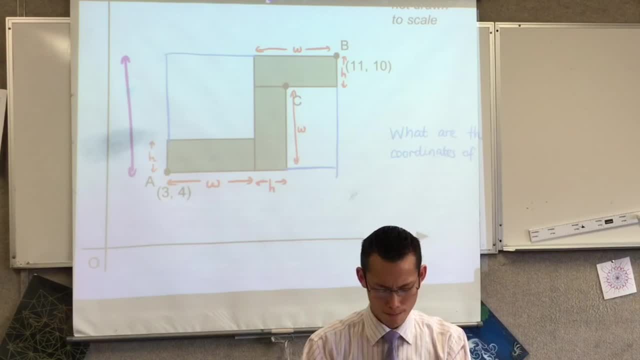 I think it's six. Now my question to you is: wait, yeah, you're looking at the other one. So six. this is up and down, right Up and down. I've got coordinates. Which coordinates are up and down coordinates? 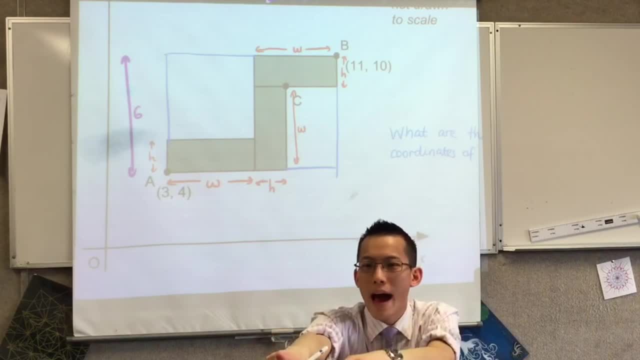 It's the. what name do we give them? They're called y's right, which is the second value. It's the four and the ten. You see that? So I've got to go climb up from four all the way up to ten. 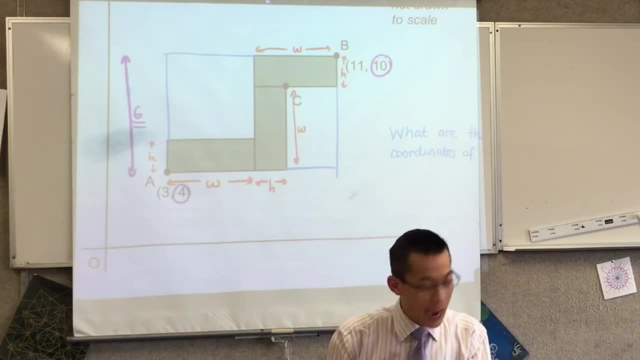 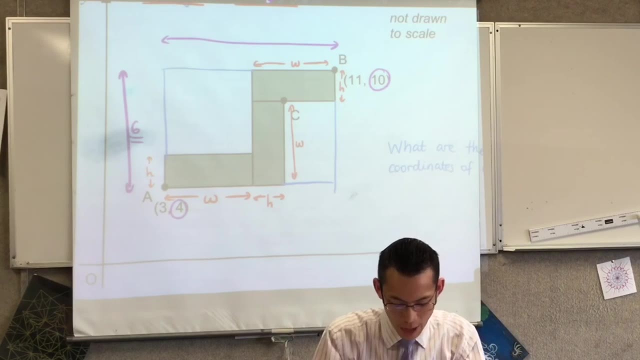 Ten and that's six. Does that make sense? Yes, Okay, I know the height. What about this one across this way? Well, you can help me out with this one, right Eight, This is eight. Okay, how do I know eight? 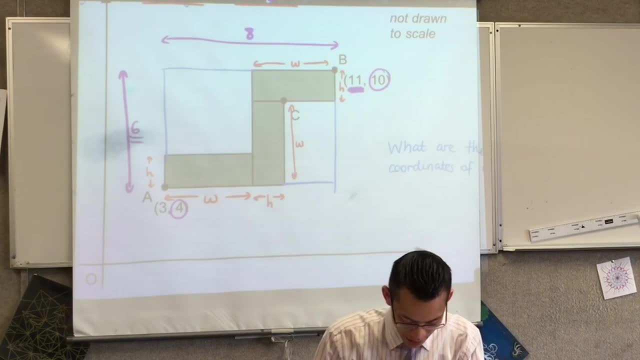 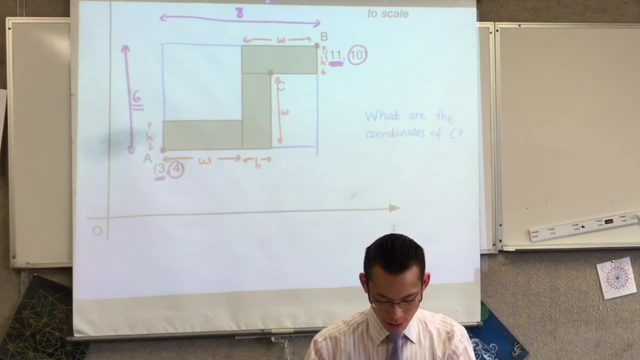 Where does it come from? Eleven, Eleven, Take away three. Okay, this is good, I'm almost there. I'm almost there. Watch this. okay, If I look up and down, right up and down, I've got w plus h. 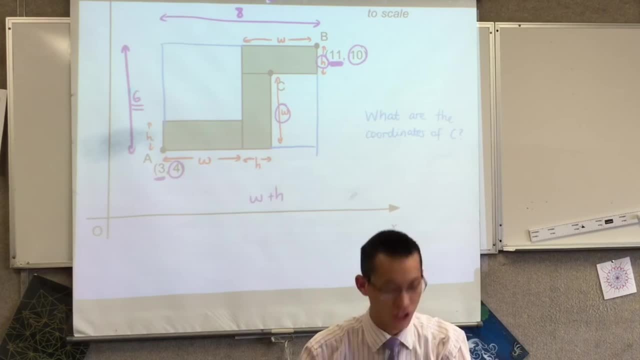 Do you see that W plus h and they're going to be that up and down length, right Six. Do you agree with that? Whatever w and h are okay. What about this width and how can I use that? 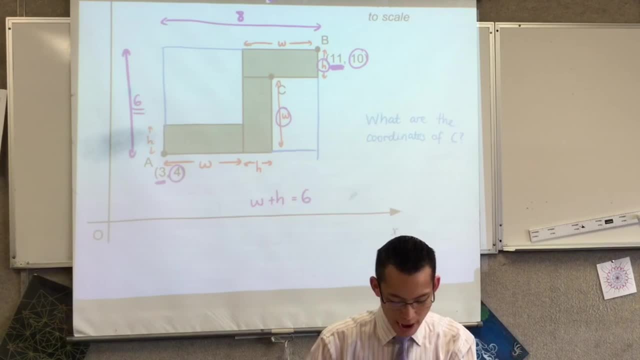 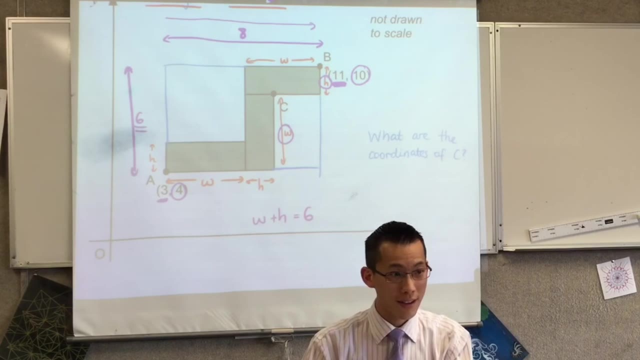 What would you like me to write? How far do I have to go, in terms of w's and h's, to go from the left all the way to the right? Can you see it? You got it. Can you see? Look, you've got to go. 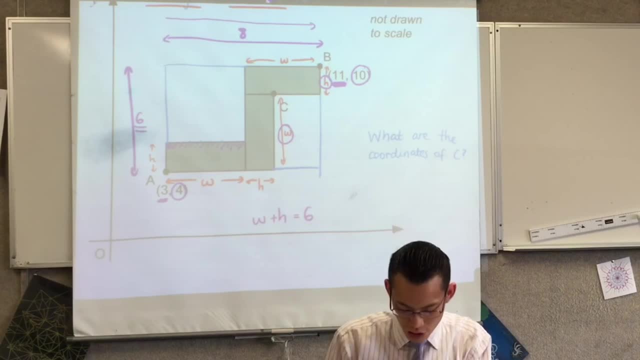 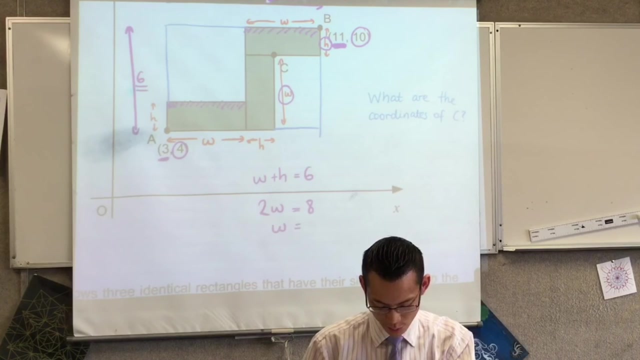 W this way, right, And then you've got to do another w to get all the way across. Do you see it? So two w two lots of w is. So two lots of w is eight. So one lot of w is four. 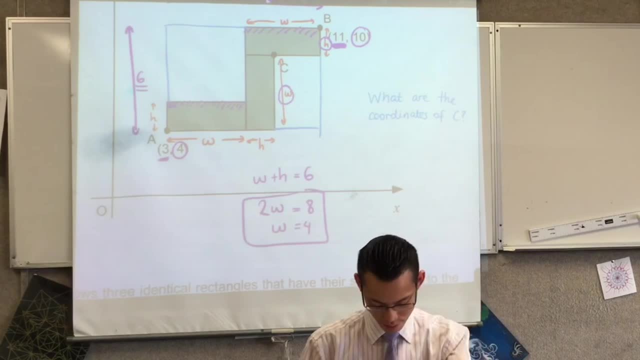 Now that you know what w is, what's h? h is two, because you can put it into here. Do you see that? So what did I do? Well, let me start again. What did we use? What knowledge did we use, Brad, to be able to solve this question? 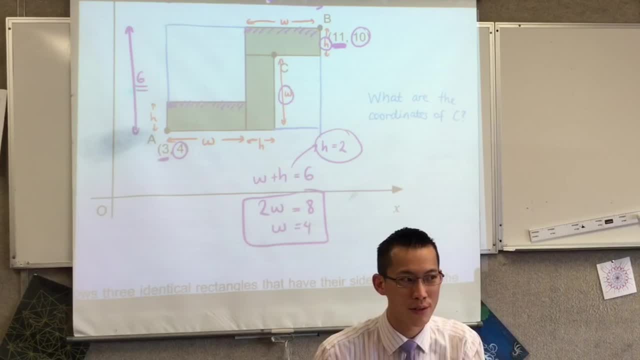 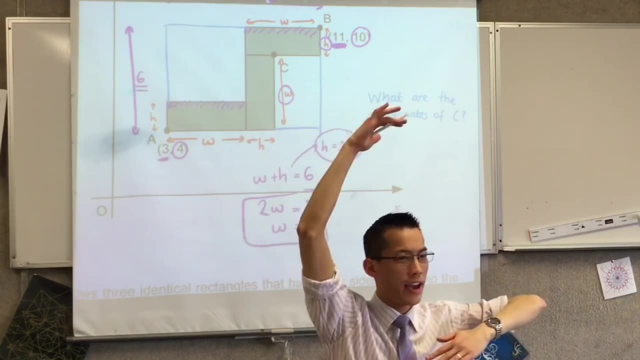 Think You all knew what to tell me to do. What knowledge did I use? I used algebra. thank you very much. What else did I use? Working with numbers. Working with numbers, I had to use the. how did I know how wide and how high? 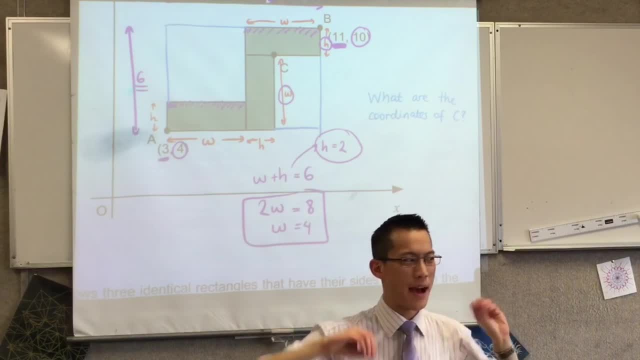 Yeah, units, coordinates, You all know these things, but I combined it in a way you didn't expect and you can do that too. Okay, All right, You can rule off that diagram. Same thing, Same thing. Oh, so I've answered the first question. 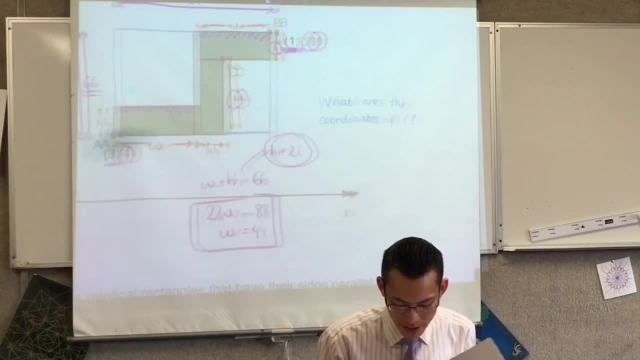 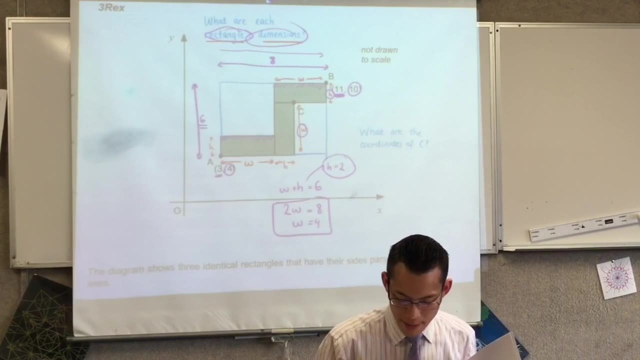 Rectangles dimensions. they're all two by four. Okay, so how do I find out where c is? How do I find out What do you reckon? Well, I've got my diagram here. Let me get rid of some of these. 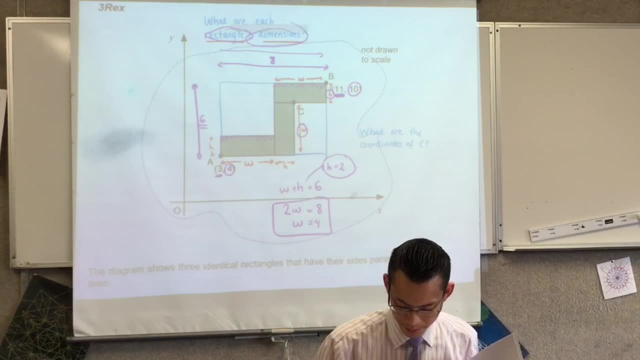 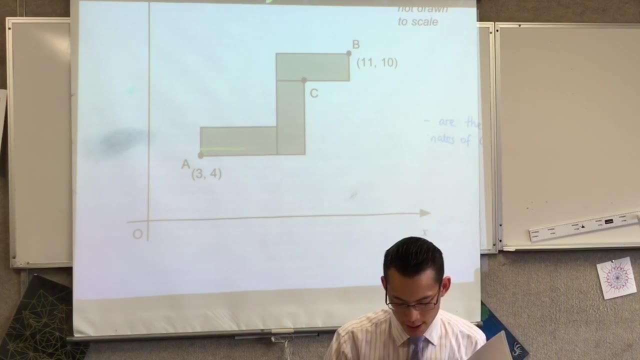 I've got so many lines here, Let me get rid of some of them. Whoops, There we go. Okay, look, I know what w and h are right, So I could, for instance, go this way: That's four. 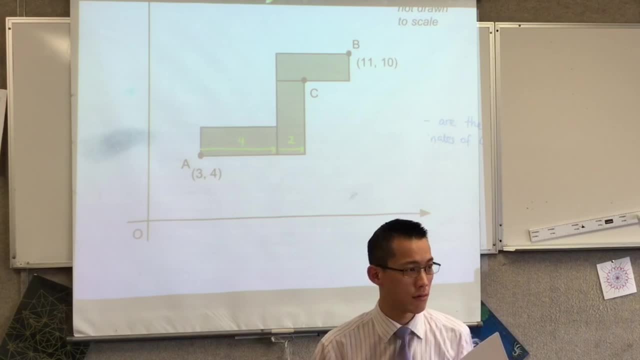 And then this way that's two. All right, So if I go six units to the right, that should give me the x coordinate right Nine, Which is nine. I got that. I got that. I got that.